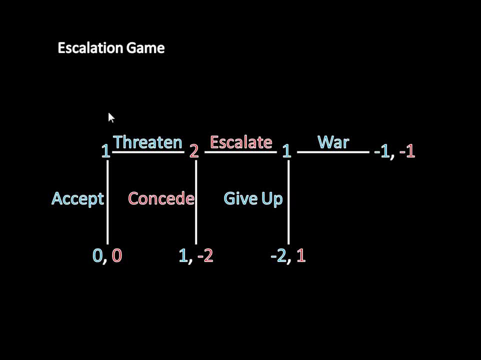 Well, you can't just randomly threaten and close your eyes and hope for the best. It only makes sense for you to threaten if what's going to happen after you threaten is better for you than if you just give up and accept right here And the only way to know what's going to happen in the future. 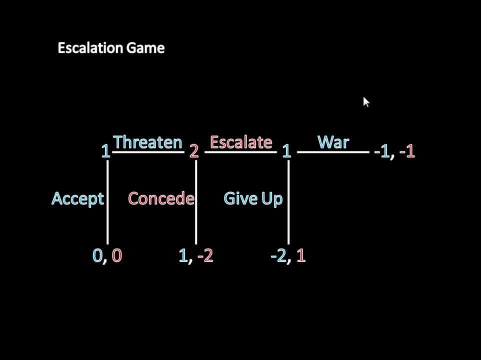 is if we look ahead into the future and work our way backward from there, And likewise for Player 2 or State 2. here it doesn't make sense for her to escalate unless she can anticipate that she'll be getting a better average outcome. 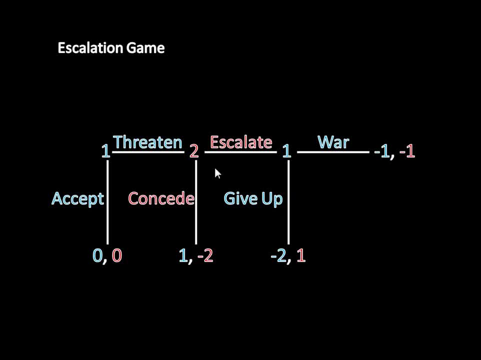 rather from escalating than from conceding. But the only way to know if it's better for her to escalate than to concede is to see what Player 1's going to do and work our way backward from there. So what we're going to be doing is we're going to be starting at the end of the game. 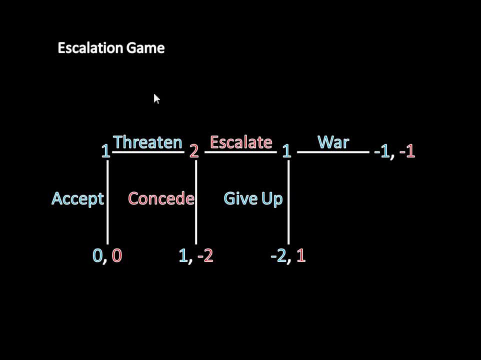 and working our way backward. So just imagine we ignore these two situations right here, these two decisions right here, and we just start with Player 1's final decision, Should Player 1 threaten at the beginning of the game and Player 2 then escalate? 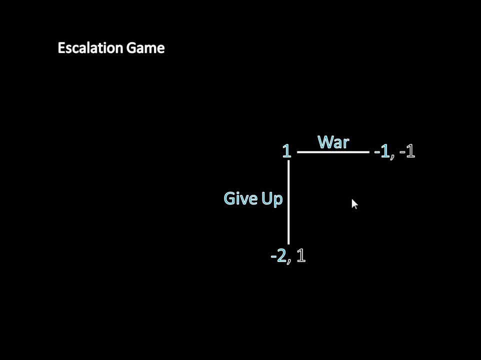 So that leaves Player 1 in this situation right here, and all we have to do is note that if Player 1's ever in this situation, war is better than giving up, because Negative 1 is greater than Negative 2.. So if Player 1 or State 1 is ever in this situation, State 1 will declare war. 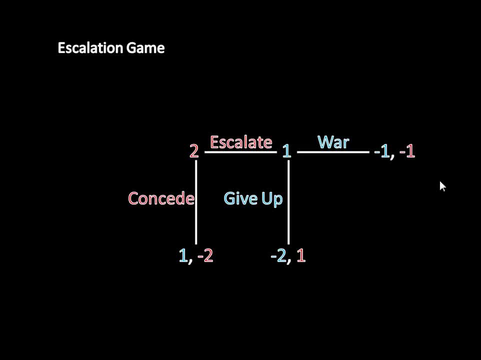 So that's that, And now we can move back a step. So now put yourself into Player 2's shoes. Well, Player 2 knows that if she escalates, then State 1 will declare war, So she can ignore this. give up decision or strategy for State 1,. 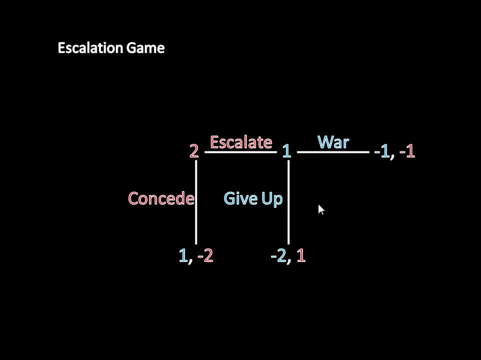 because State 2 knows that State 1 isn't going to choose that. So essentially, State 2's decision looks like this: This give up thing isn't here, because she knows that State 1's not going to give up, State 1 is going to declare war. 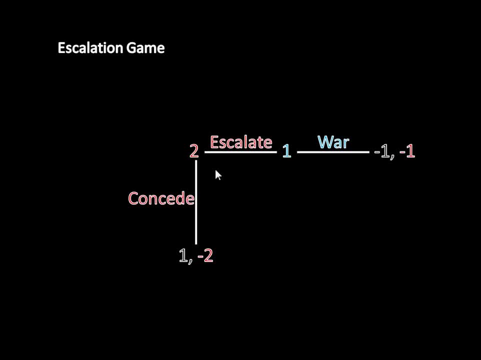 So in that case, if State 2 concedes, she gets Negative 2.. If State 2 escalates, State 1 declares war and she gets Negative 1.. Since Negative 2 is worse than Negative 1, it makes sense for State 2 to escalate. 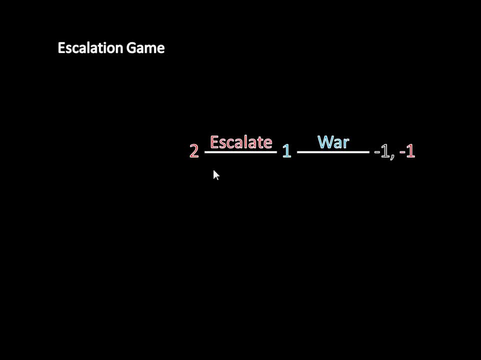 So if State 2 is ever in this situation, she's going to escalate, And then that's that. So now we can just move back to the original decision and we'll be done with the game. So State 1,, instead of looking at this complex situation, knows that in the future, if he